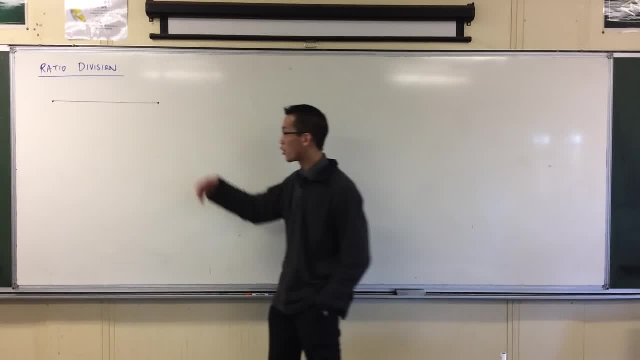 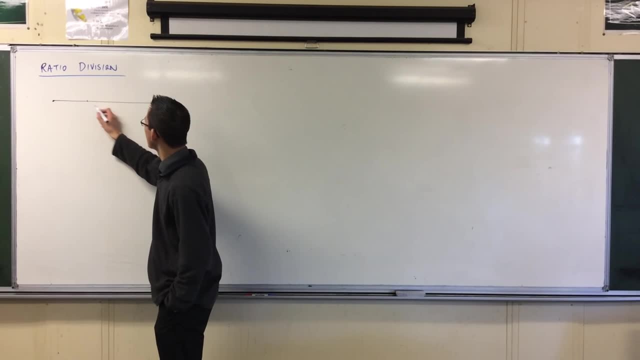 We've already established all of that. So now I just want to get at the idea of if you've got an interval, in what ways can you divide it? So if I said, okay, let's divide this interval into three equal parts, 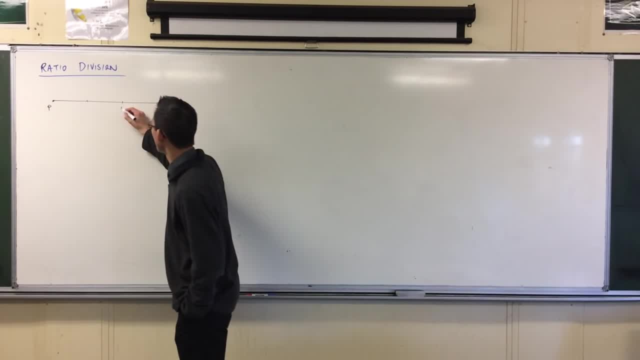 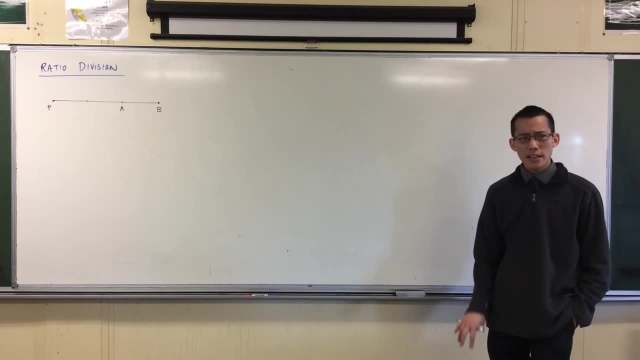 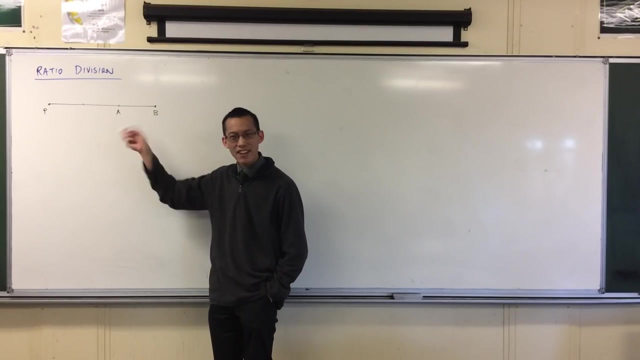 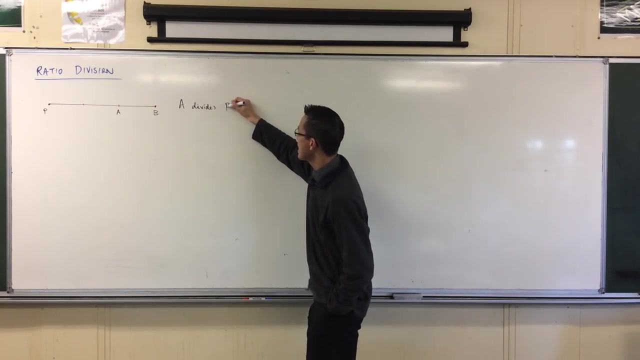 And if I label some of these points like so Okay, Now, being that these are three equal parts, I can say that there's this interval pb, right Here I can say that a divides pb. Now they're three equal portions. 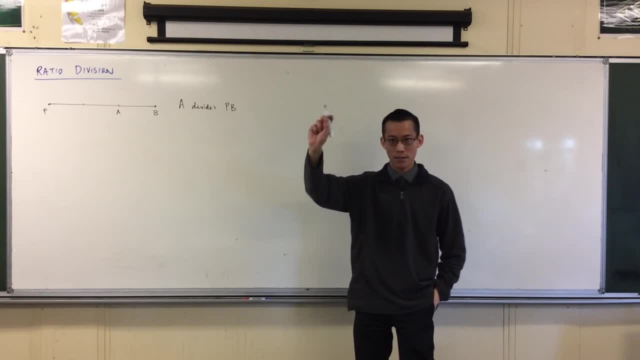 And I've said pb, which means I'm starting from the left and going to the right. okay, So what ratio is it? It's 2 to 1, isn't it? It's 2 to 1.. Isn't that the evacuation room? 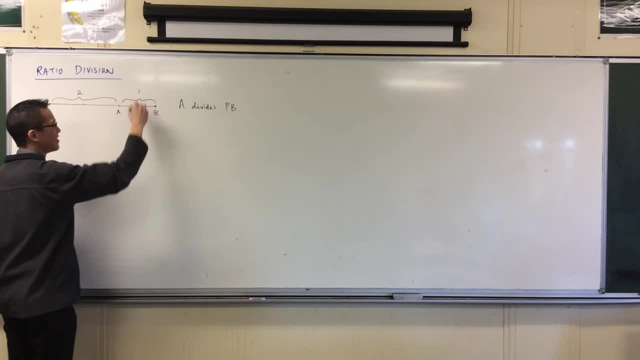 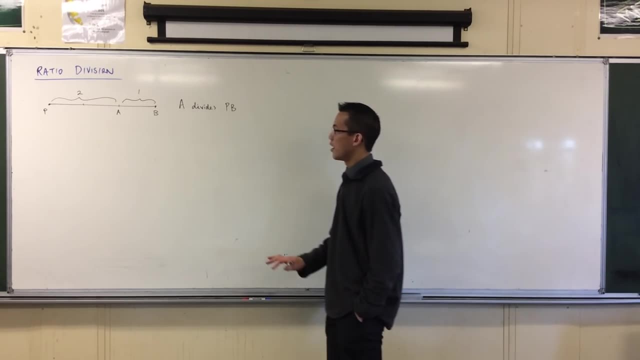 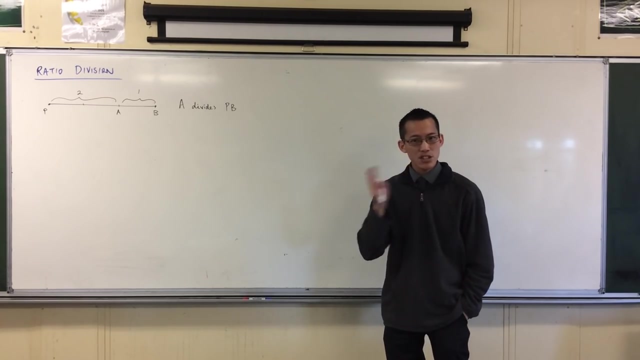 It's an old bell room. Doris looks so excited Now. a divides pb in the ratio 2 to 1.. But I'm going to add in a little more detail on this because you see where it's going. It doesn't just divide pb in the ratio 2 to 1.. 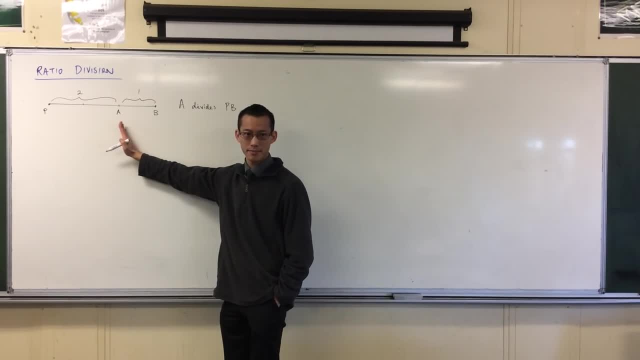 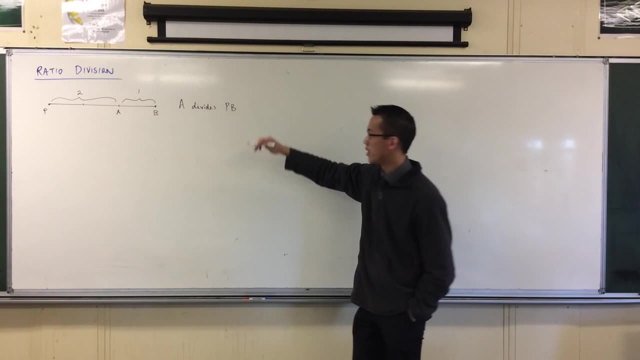 It divides it internally in the ratio 2 to 1.. Because a is on the inside of pb, That makes sense. How else can you divide it? But I want to get this word down right. So a divides pb internally in the ratio 2 to 1.. 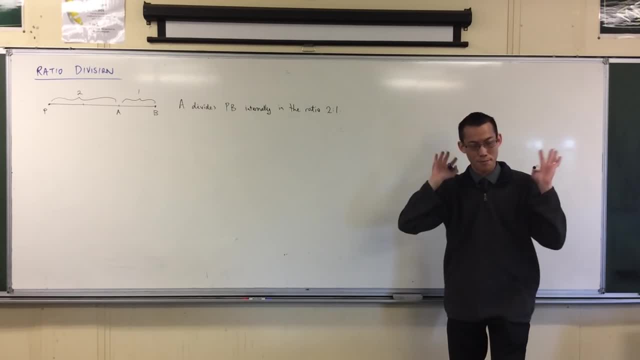 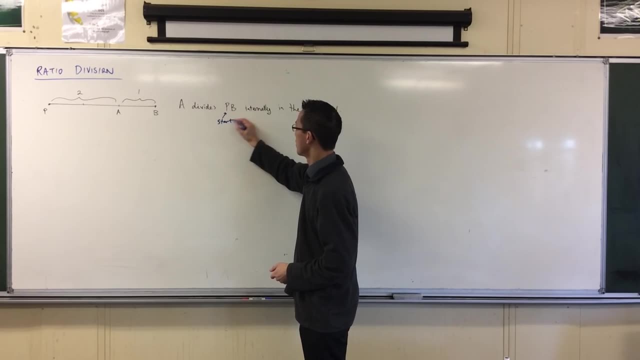 Okay, Maybe you want to make a note. I'm trying to make a beat out of this, because so many students get confused about it. Now, pb means start here and end here, right? Not just pb, Not just alphabetical, all the time. 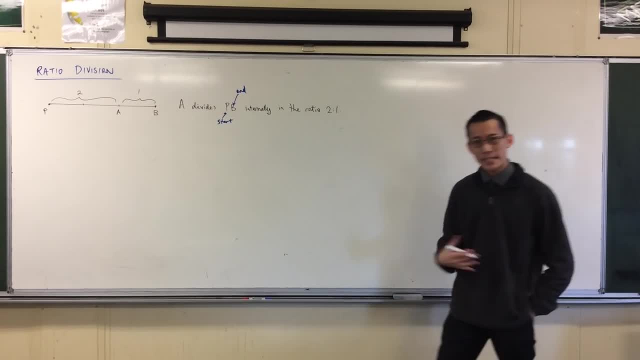 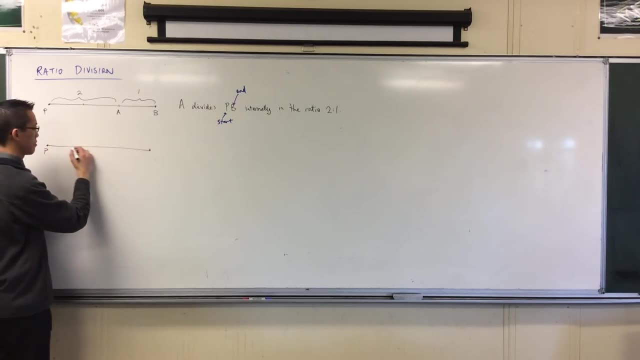 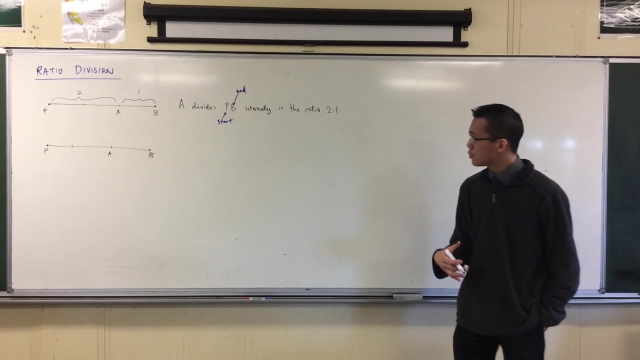 You really got to pay attention to the way they give it to you. Okay, But in the same way, if we just copy this diagram again, same set of points, same set of ratios. Okay, I've used pb as my interval, right? 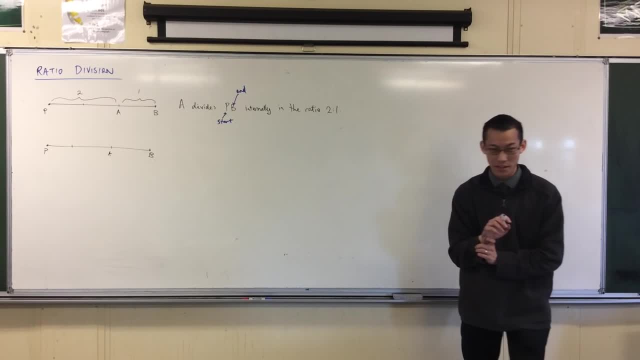 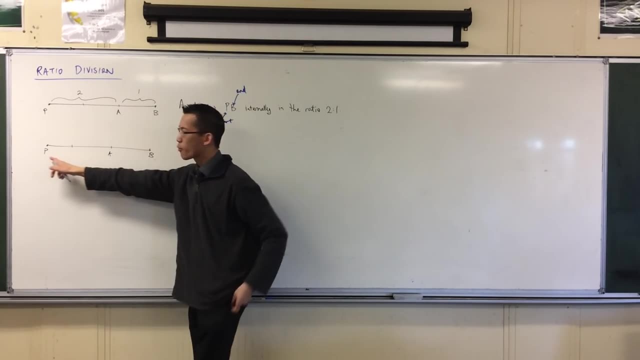 But it's not the only interval on there right, In fact, there's at least two others. So I could say, for instance, instead of a dividing up this interval, I could talk about p dividing this interval. Now, that's a bit weird. 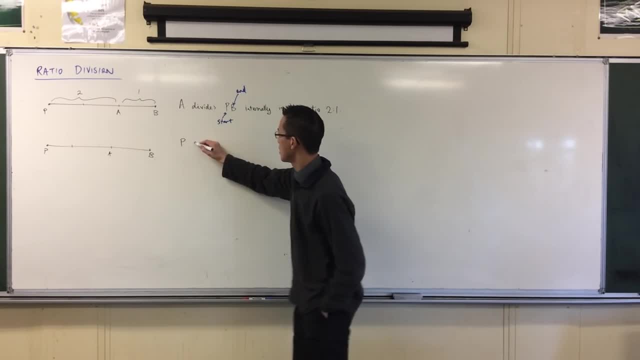 It's a little bit weird, But let me show you how it works right. p divides ab Now, unlike a with respect to pb, when we think about p with respect to ab, p is on the outside, p is on the outside. 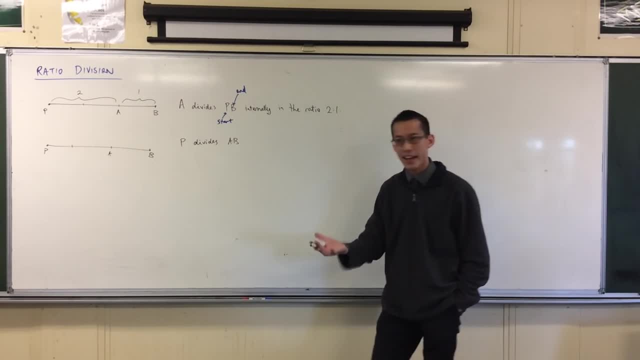 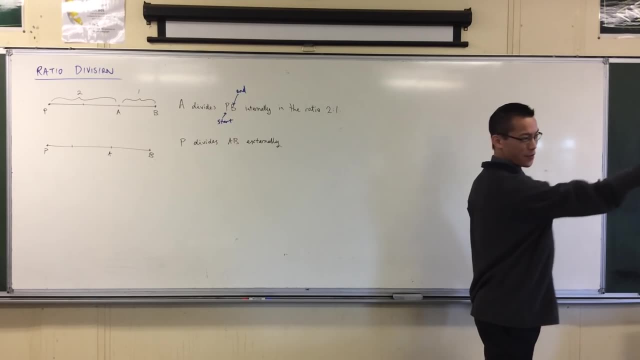 So it's not dividing internally, It's dividing externally. That's a kind of strange idea, right. Right, Like if you had a pizza and you said, hey, divide this up, And you're like I'm going to cut over here on a different table. 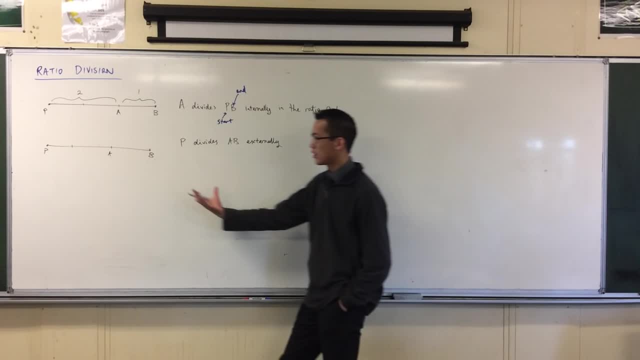 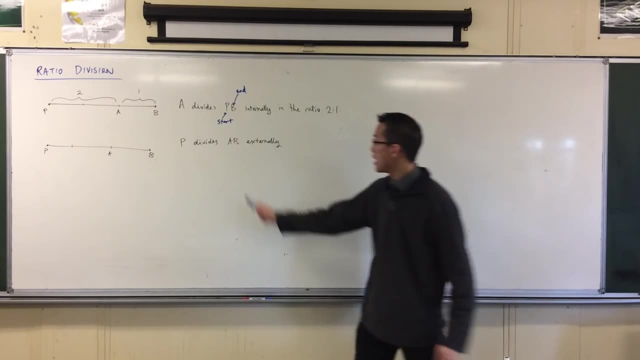 That's weird, okay, But it's getting the same idea that, look, there's still division of intervals. okay, It's just going another way. Now, remember I said that pb means start at p and end at b, right. 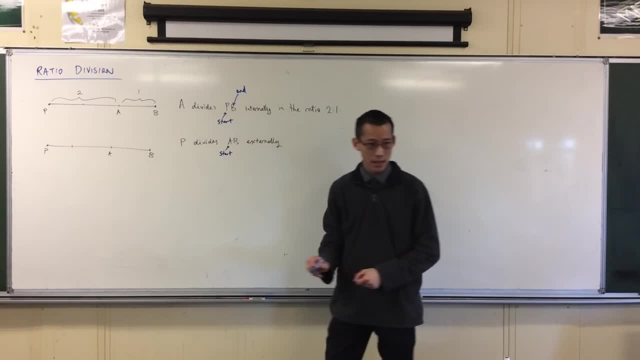 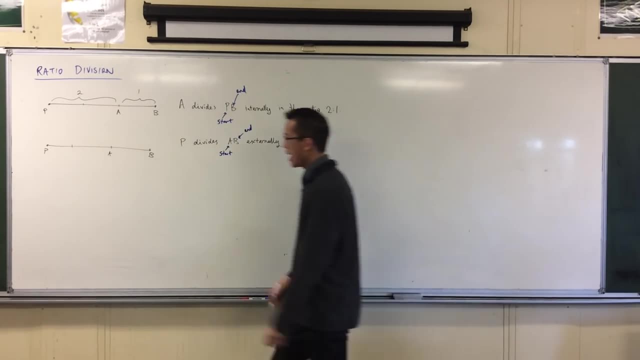 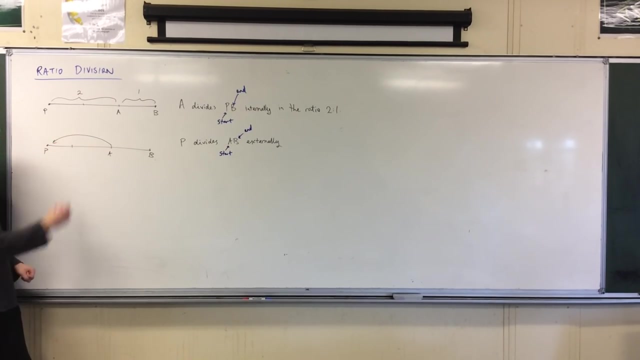 So it's the same thing here. You start at a and then you end at b. Now how would this work? How would this work? Answer? If I start at a right, I have to go outside this way to get to p. 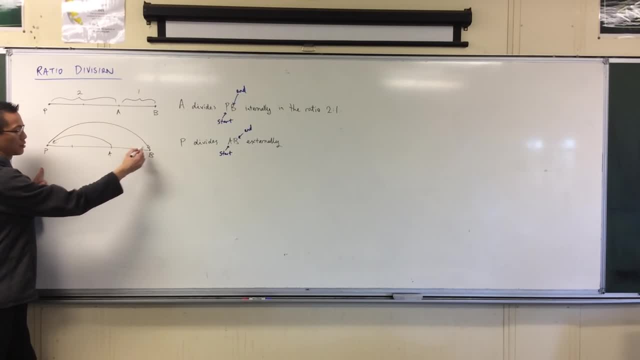 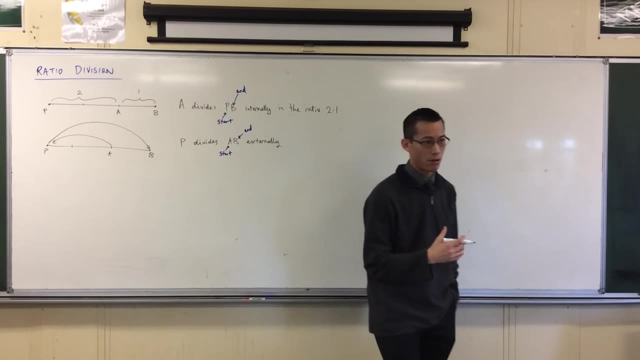 And then I have to go the opposite direction to get to b. okay, Now have a look at these two arrows that I've just drawn right. What ratio are those two arrows to each other? Yeah, Negative 2 to sorry 2 to negative 3.. 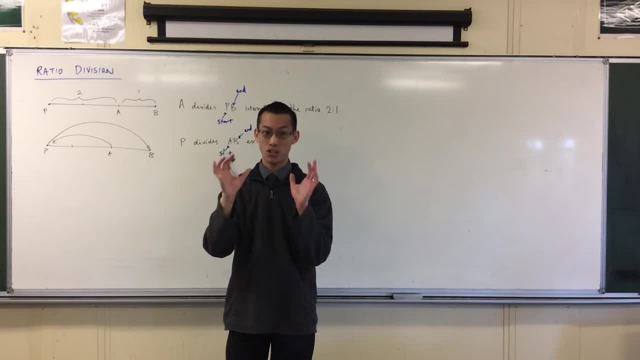 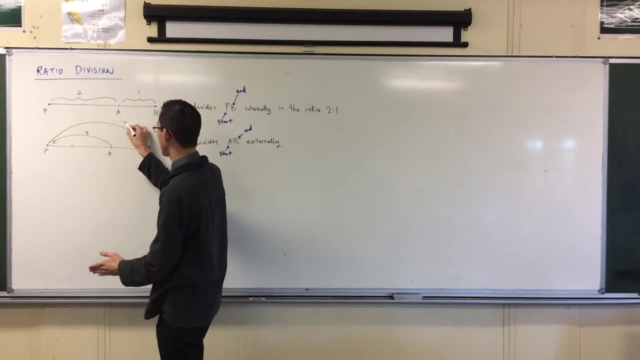 Okay now I can think about this in a couple of ways. If I just think about them as lengths, just think about them as lengths, then this is two portions, right, And this is three portions. So it's 2 to 3, okay. 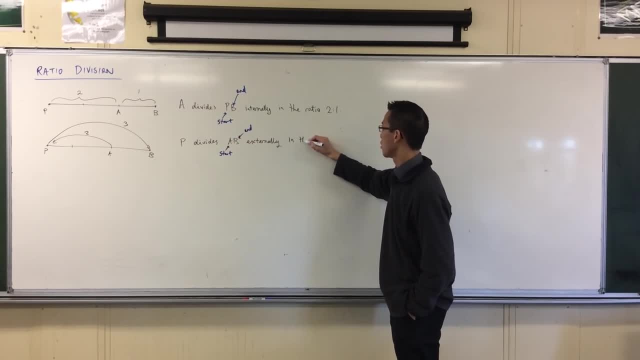 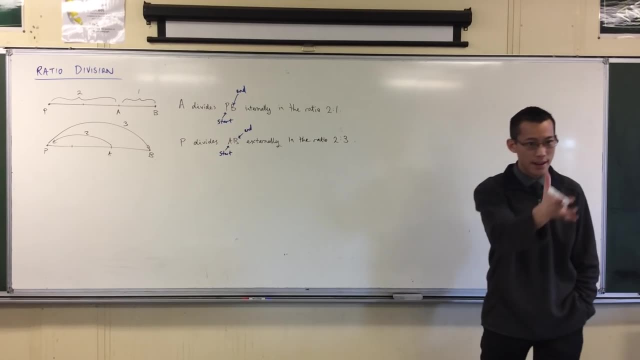 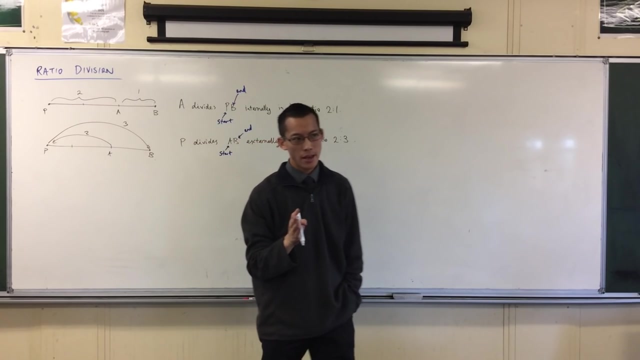 So I can say, divide ab externally in the ratio 2 to 3, okay, But as you've noticed right, and this is why I put arrows on here- these are going in different directions. They're going in different directions. Not just that, but if you said, okay, let's have some coordinates for a and b, 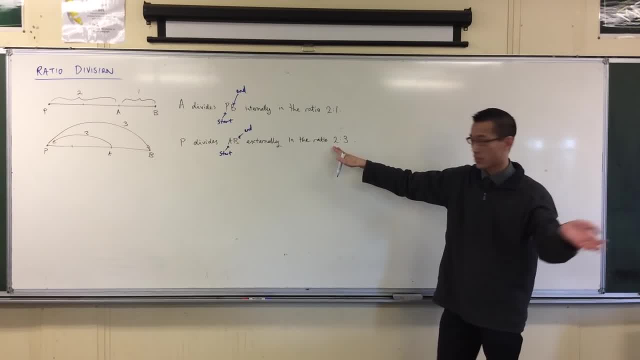 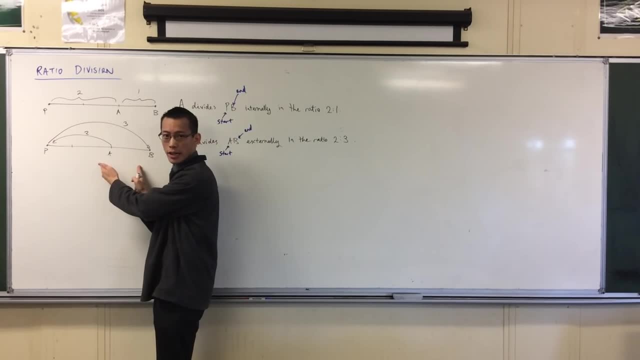 Here's a ratio Right. Pop in your k and your l and so on. If you gave that a go and just crunched this into your formula, p would end up in here, wouldn't it Right? In fact, 2 to 3 inside there means you've got to divide this up into one. 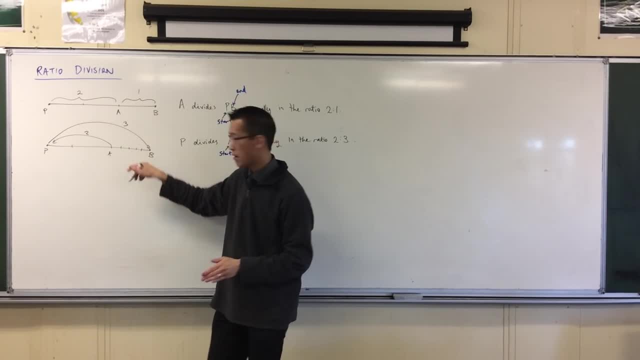 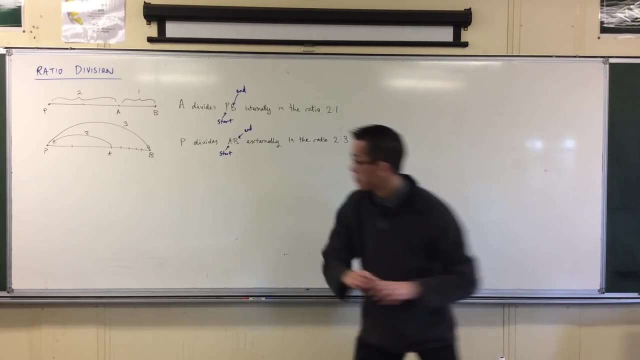 two, three, four, five components in there right, And then let's get a different color, And then what would happen is that's what I want. 2 to 3 means you go 2 first and then you go 3.. 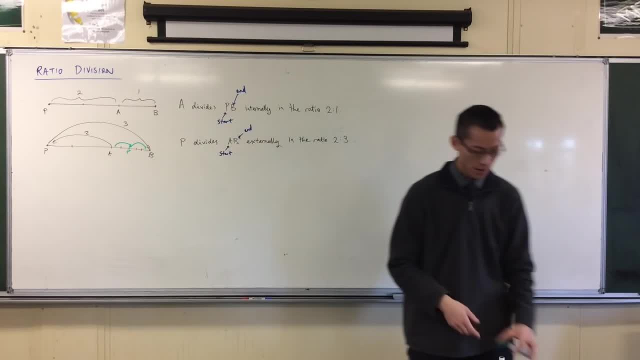 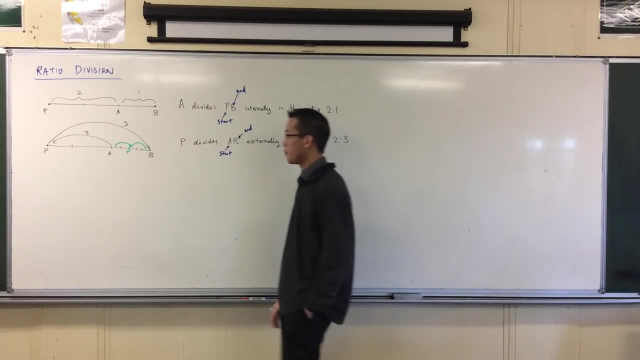 So that's where p would be. We don't want it to be there, right? So, therefore, to account for this and use the same formula, right? there's one of two ways to do it. You can think: alright, I'm going outside first. 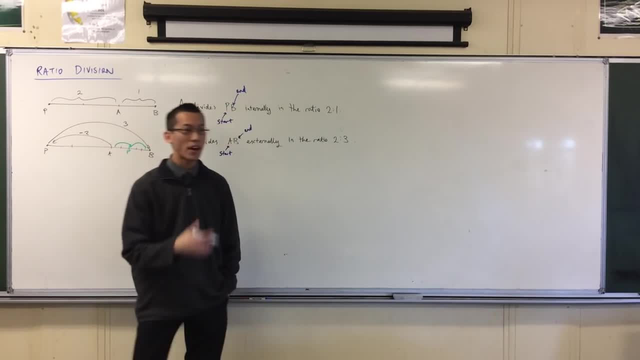 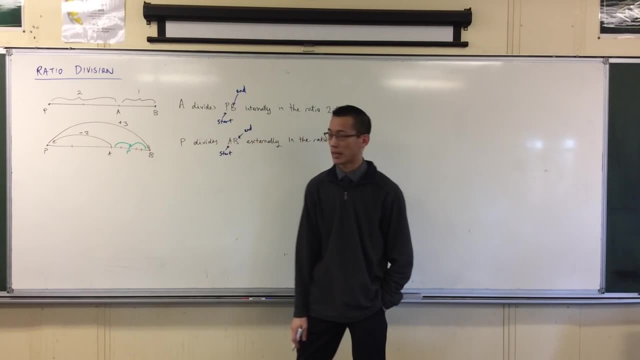 I'm going outside, So I'm going to call this negative. 2. It's going away from b, okay, And then I'm going to go plus. 3. They're just opposite directions, That's all okay. So that's one way to think about it. 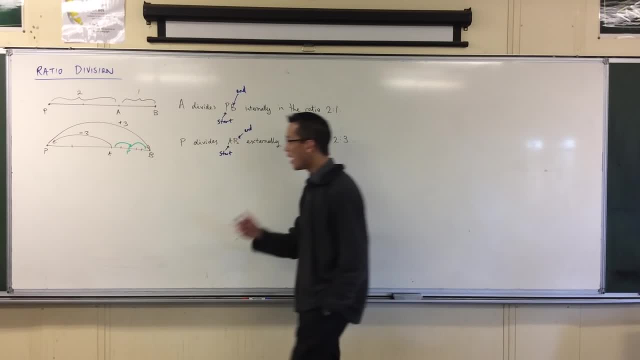 That's the way that I prefer personally, But you can think about this from two different angles. I'm going to draw one more copy of the interval and I'd like you to do the same, So I've got the same p, a and b. 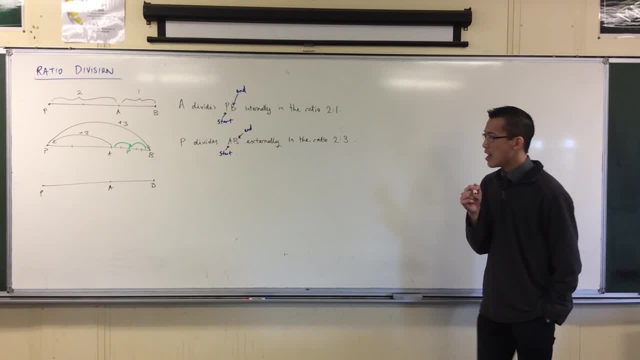 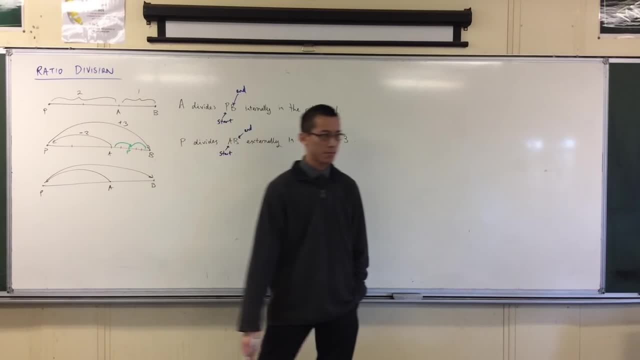 Hmm, okay, If I'm saying I've got a, I've got to start at a, I've got to go out here to p and then go over here to b, right, There's nothing stopping me thinking about these in terms of: well, let's just call this one. 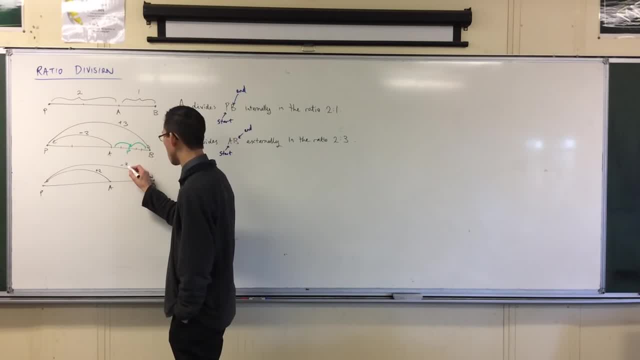 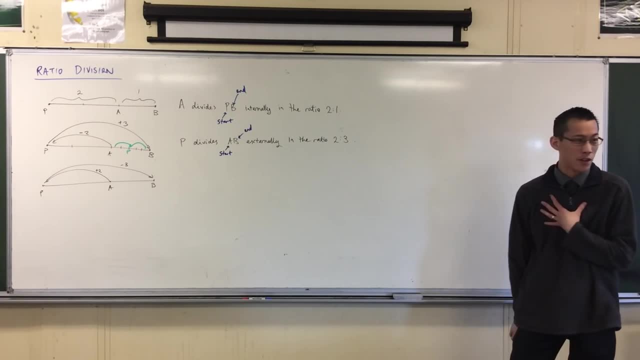 forward, which will make the other one backwards. okay, Because they're in opposite directions. Now that might weed you out a little bit, because it weeded me out a little bit when I first discovered it. because ratio division of all of the formulas- 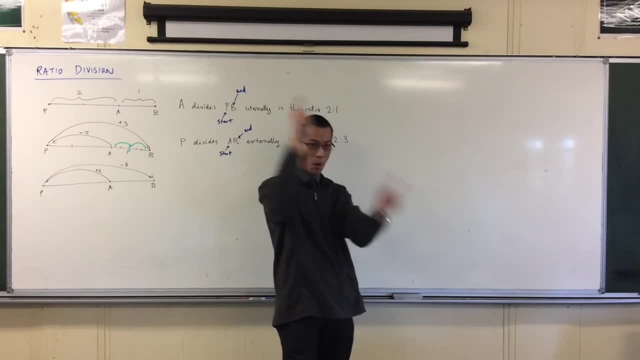 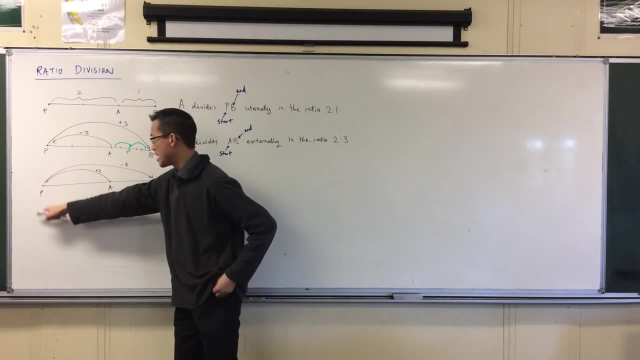 is the one where it's like order really matters. Don't just like swap things around, You'll get something different. okay, And the thing is we haven't swapped any numbers. This isn't 3 and then negative 2.. 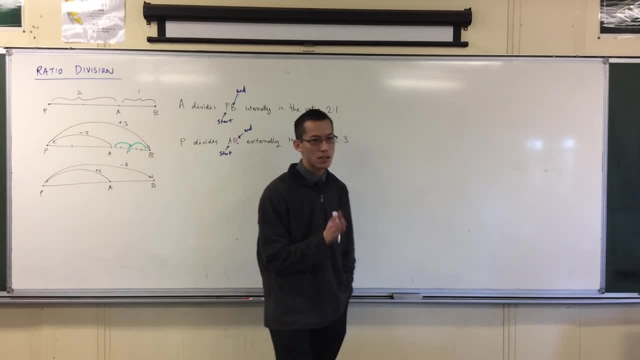 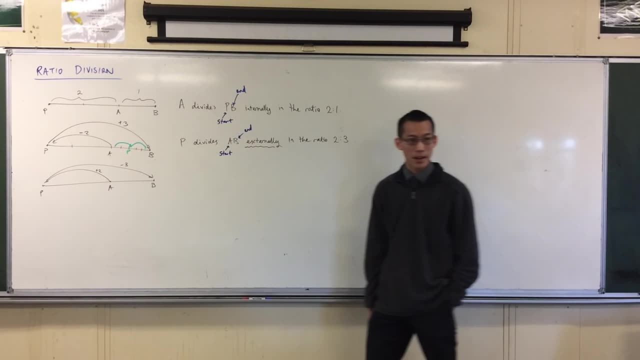 That wouldn't work. okay, We swapped the signs Now to satisfy you that this actually works. here's what this means. okay, When you see the word externally. okay, what that's telling you is: one of these numbers is going to be negative.